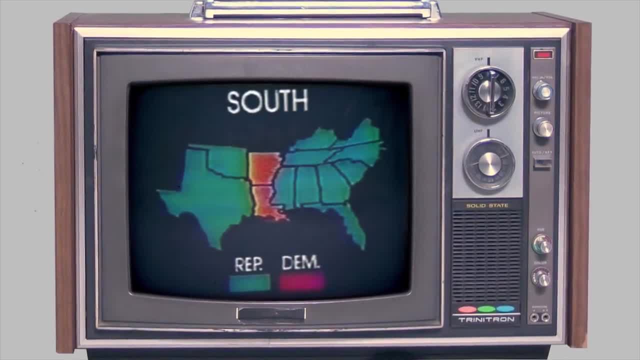 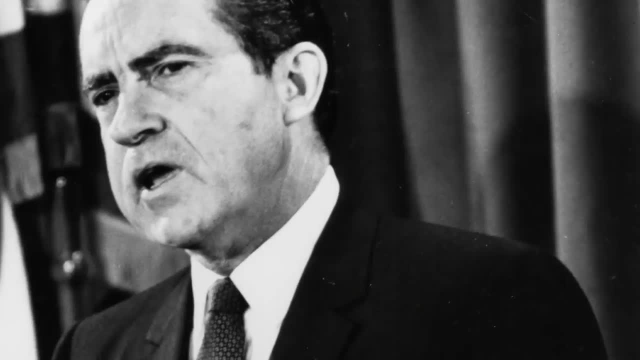 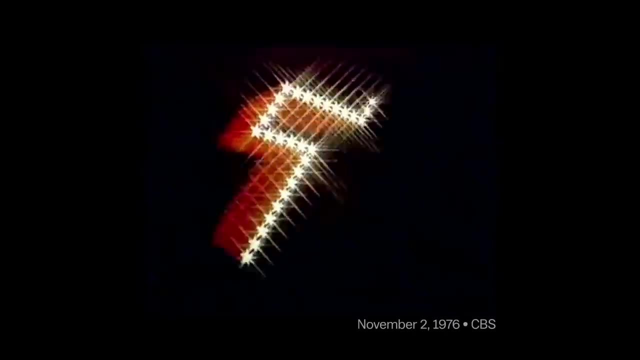 conservative state. It was colored pure Republican blue. No, your eyes were not deceiving you. The states that Republican Richard Nixon won that night in his 1972 landslide victory were colored blue on the CBS map. CBS's great broadcast innovation would soon inspire the other networks to introduce 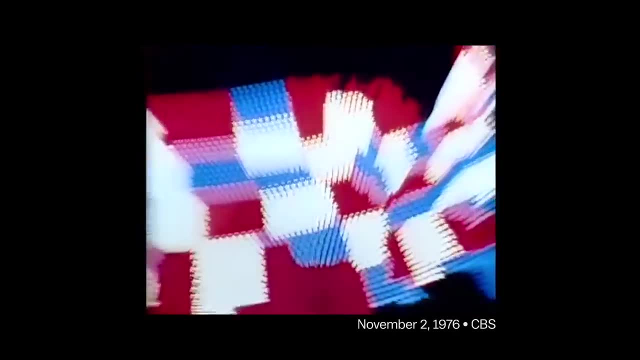 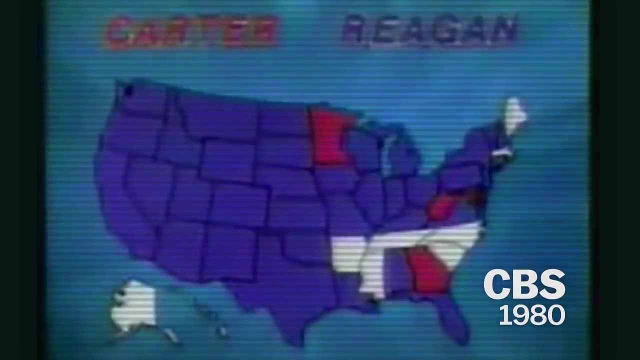 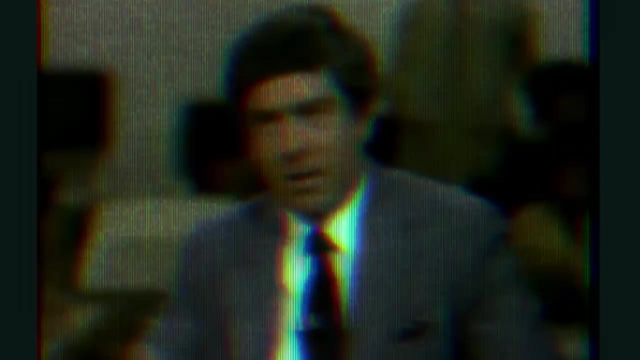 red and blue maps to their own election night broadcasts. For its part, CBS would keep the Republican blue and Democratic red scheme through the 1980 election. For Reagan it was a different story. They're shown in blue and this country is almost solidly in the Reagan colors tonight. Those 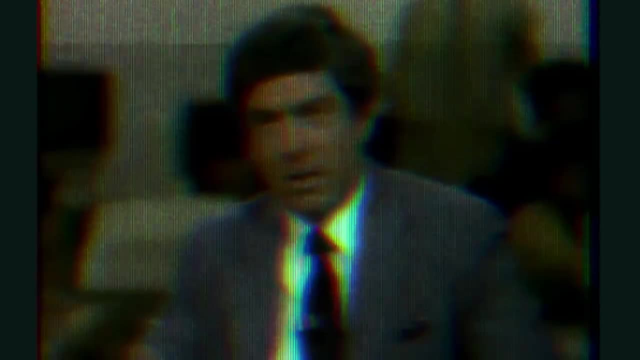 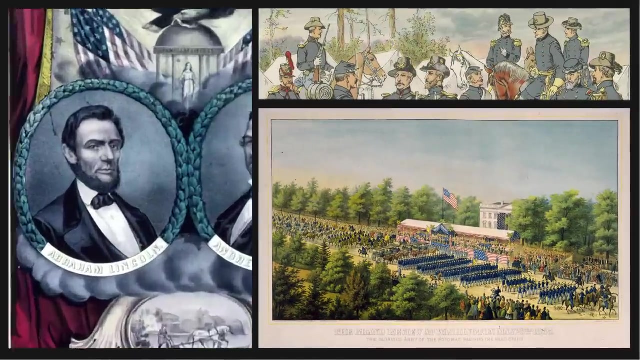 pairings may seem odd today, but they weren't back then. That's because blue, as NPR's Ron Elving has noted, was a color closely associated with the Union army led by Republican Abraham Lincoln. Red, on the other hand, was a color associated with leftists and left-leaning parties throughout. 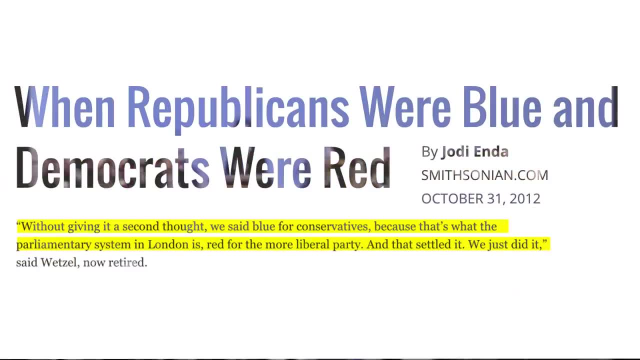 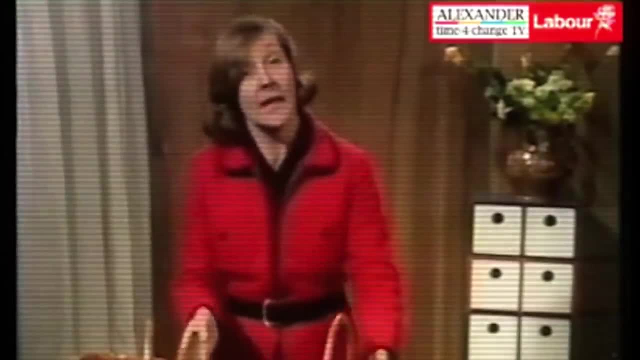 the world as it is today. In fact, NBC's 1976 election chief told the Smithsonian magazine that it was British Tory blue and Labor Party red that influenced NBC to go with this color scheme for 20 years. You can see it looked like a suburban swimming pool over there, Walter Mondale. 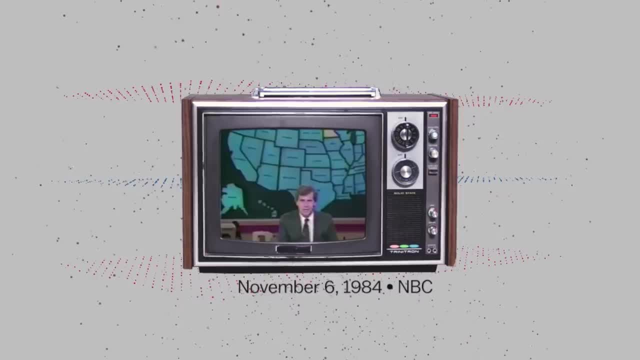 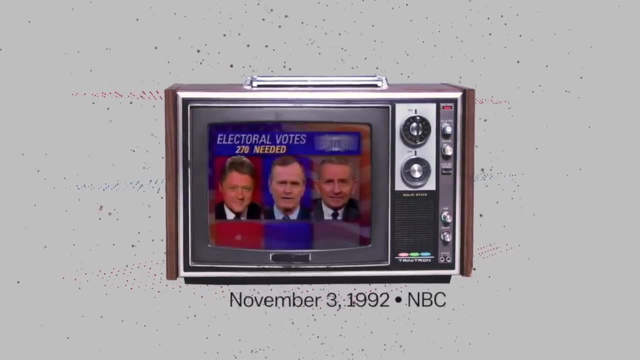 the winner of the state of Minnesota, colored red, which is the color of the state of Kentucky. It is shaping up as a George Bush map as we look at it back there. It certainly is, Tom. He goes into the Clinton column after having voted with the. 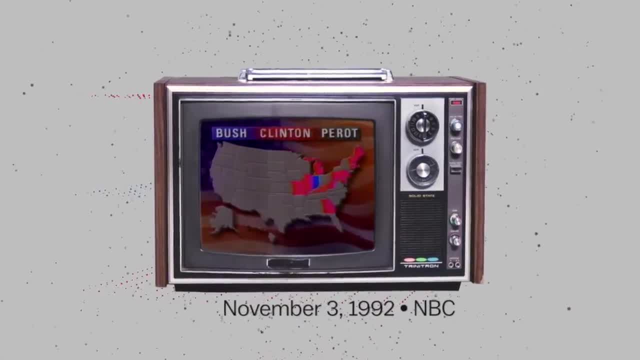 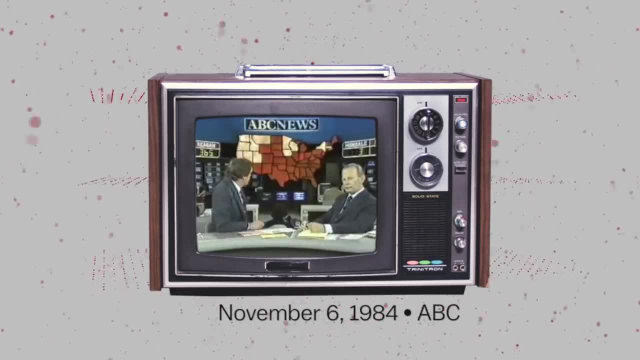 Republicans the last three times And, as you can see, we color in the state of Kentucky. ABC News, on the other hand, had its own state color logic. Red states are states that we have projected. having gone for Mr Reagan, Red are Reagan. 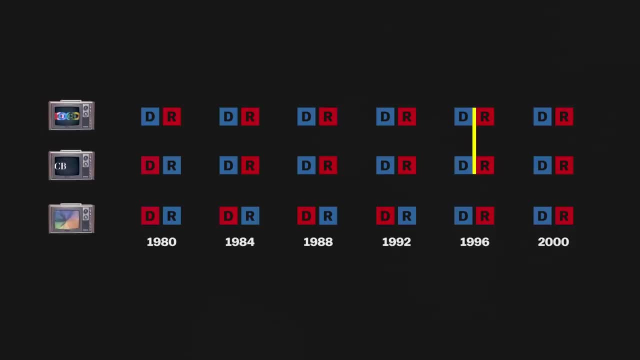 That's why we chose red. By 1996, ABC and CBS had used the now-familiar Democratic blue states and Republican red states on their maps over several election cycles. So NBC decided to make the switch too, for a very simple reason. 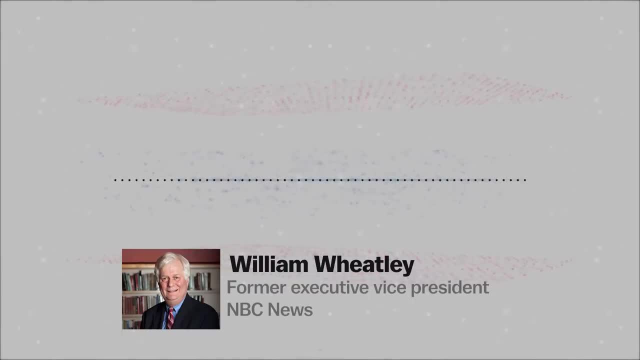 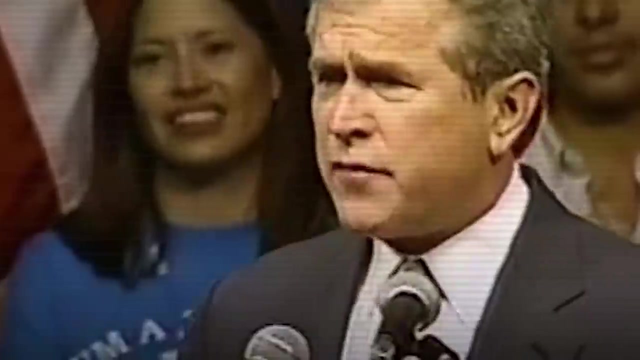 NBC decided to adapt the same color pattern as ABC and CBS so as not to have a confusion for the viewers. But it wasn't until the 2000 election that the political concept or term, red state versus blue state took hold On that election night. 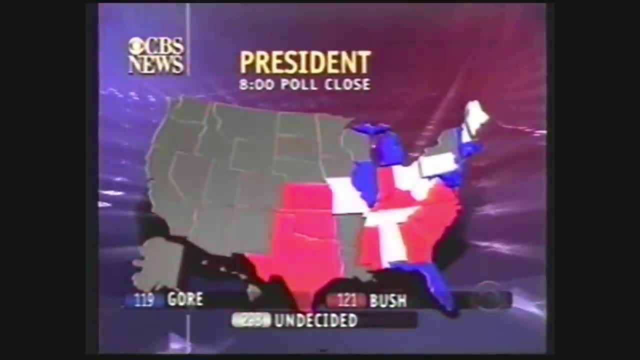 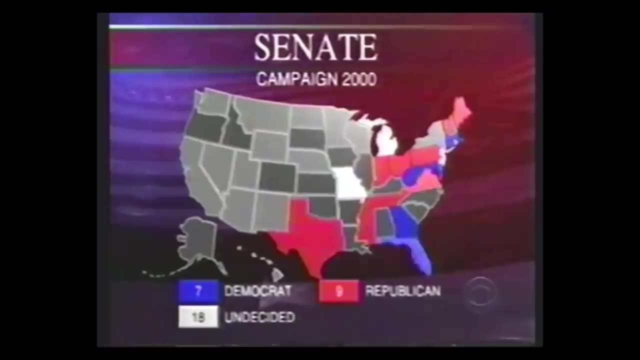 network anchors and pundits relied heavily on the colored maps to explain how close the race was between George W Bush and Al Gore. Very soon, those red states and blue states that the country saw over and over again on TV became rooted in American culture. David Letterman was one. 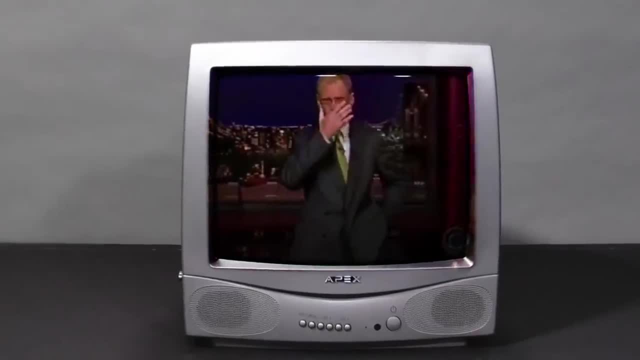 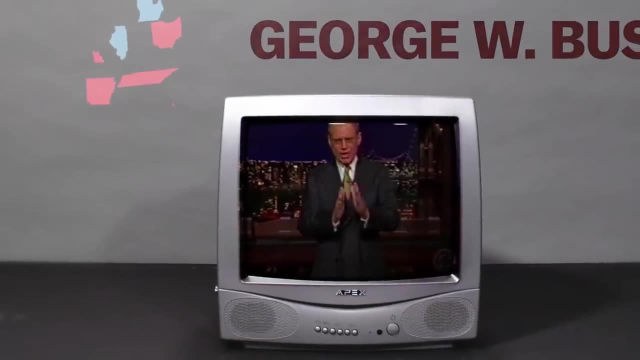 of the earliest cultural figures. to pick up on this, just a few days after the 2000 election, Candidates have worked out a compromise and, thank God, not a minute too soon. Here's how it's going to go: George W Bush will be president for the red state. 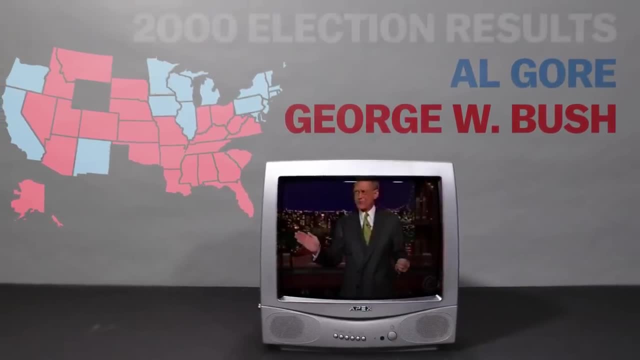 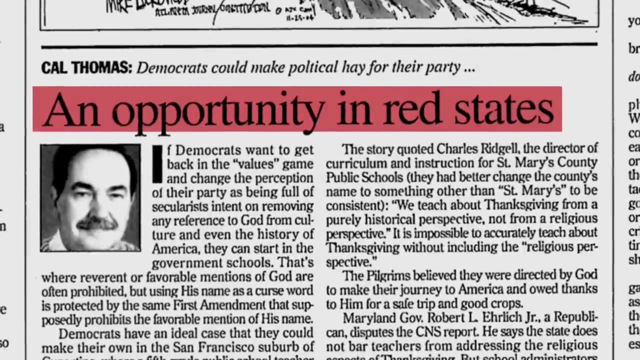 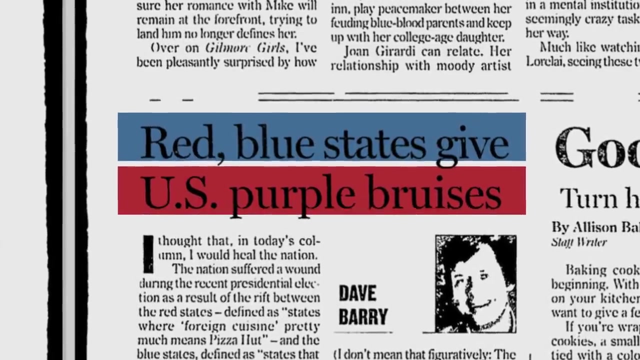 Al W Gore will be president for the blue state. Those same television maps would also help make red state and blue state a popular term among political pundits and newspaper headline writers. It was useful shorthand as memories of the 2000 election were burned into the American psyche. Over time the term came to mean not just the 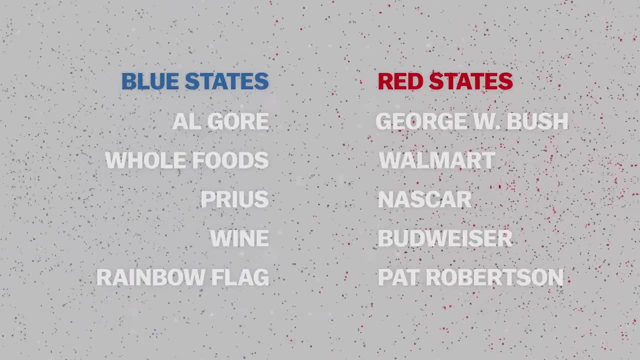 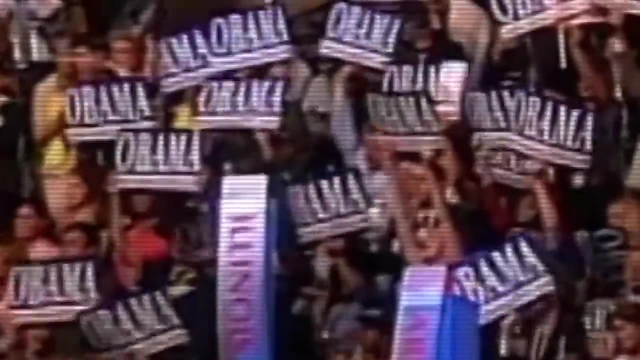 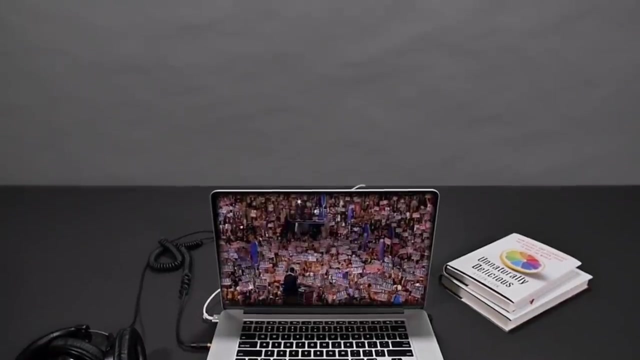 states that voted for Bush and Gore, but also a way to describe the cultural values associated with electoral geography. All this was not lost on then-state Senator Barack Obama when he addressed the DNC in 2004.. The pundits- the pundits like to slice and dice our country into red states and blue states. 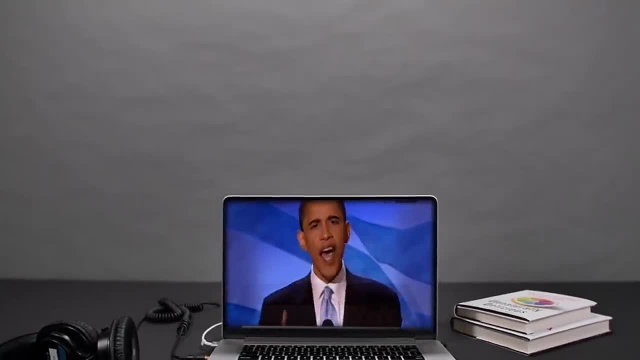 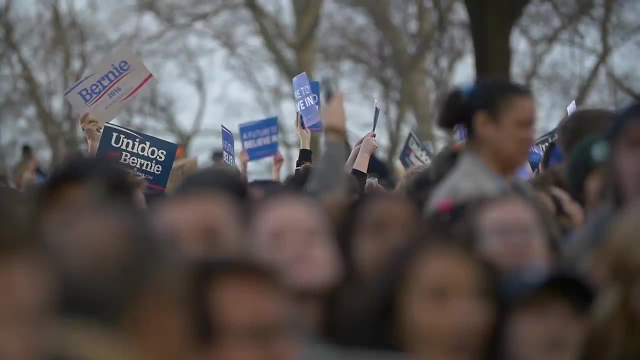 red states for Republicans, blue states for Democrats. But come election night in 2004,, the term, the coloring and the maps still stuck. Now you can see the red and blue terminology all over the place in American life. It's in modern. 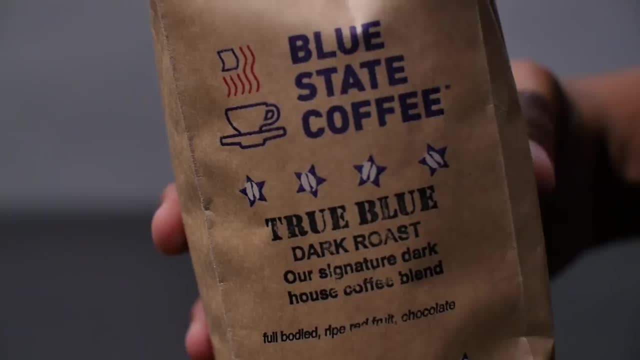 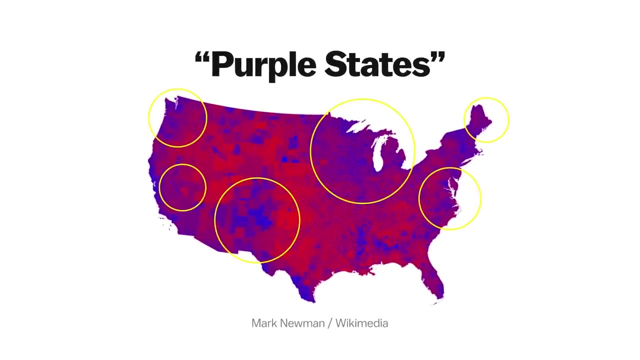 geography, it's in the names of consulting groups, in coffee brands and even at this Kentucky barbecue joint, There's even a color now for states that could vote: either Democratic or Republican. And while many may lament the divisions that the terms have brought to the 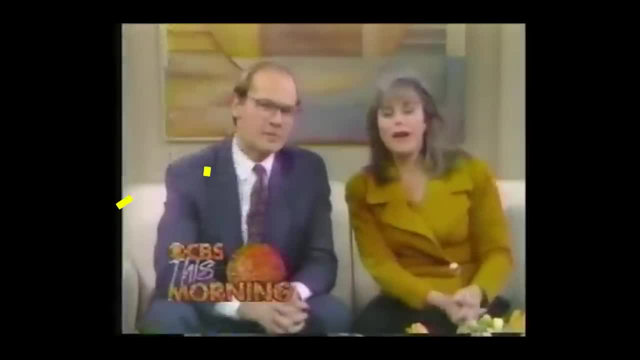 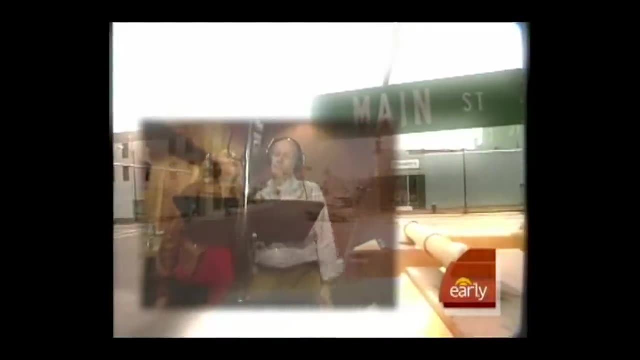